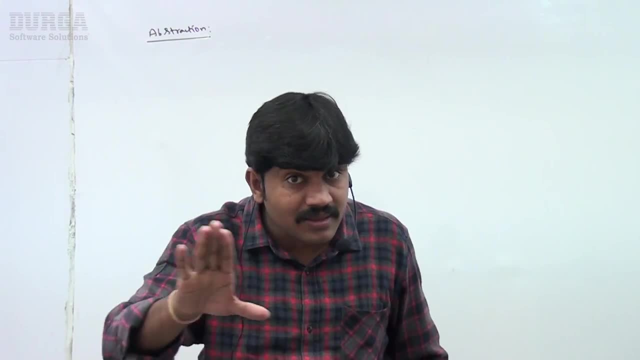 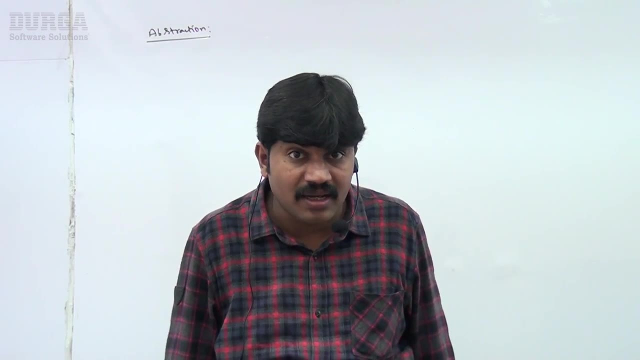 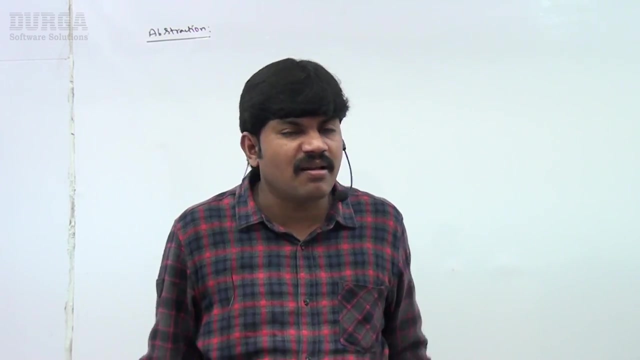 So something like abstract means not complete, not complete. In the last session, somewhere we cover an abstract class. Have you remember right? Abstract class? Abstract class means partially implemented, not completely provided class, Partial, partial, that is not complete. 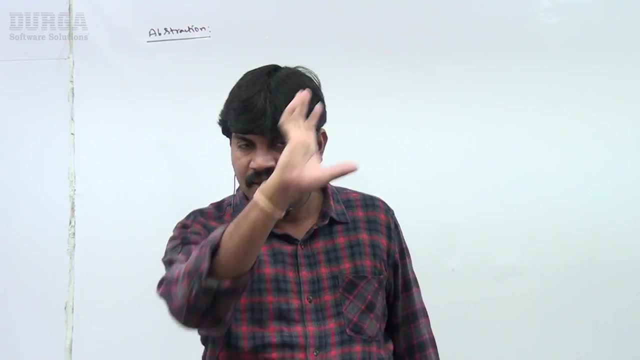 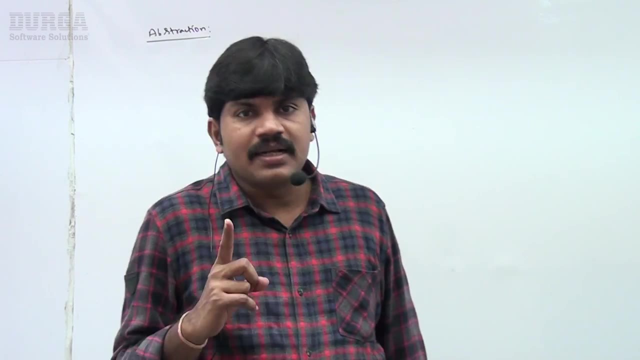 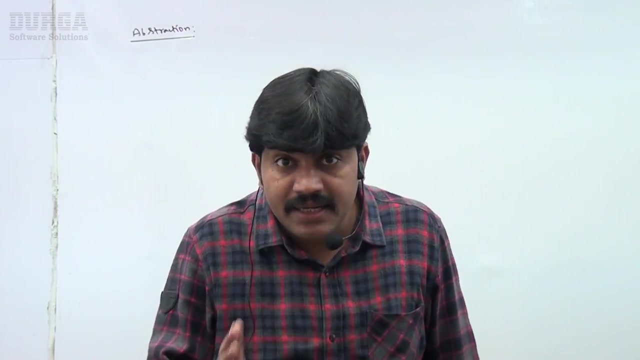 Partial type of body is nothing but abstraction. Okay, Well, sir, in the whoops, sir, which feature is called abstraction? Very simple, sir: Hiding internal implementation. Hide, hide Internally how it is implemented. Hiding internal implementation. Just highlight the. 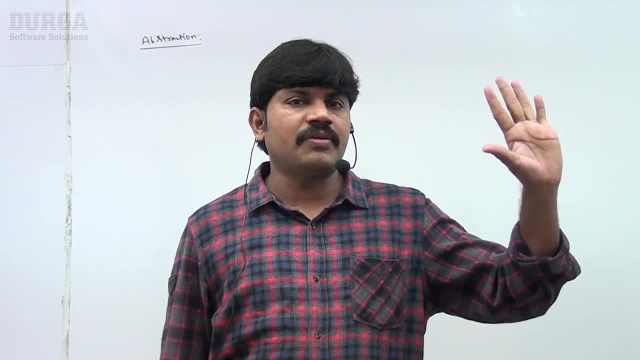 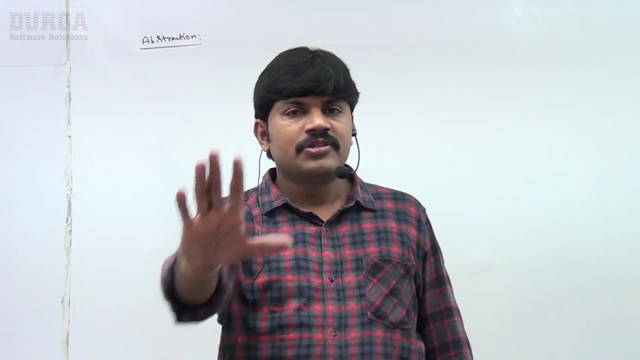 set of services, what we are offering, Sir, these are the services, what I am going to offer. So I am going to tell that. But how internal, Internally, these services are implemented? Sorry, don't ask security reasons, I don't. 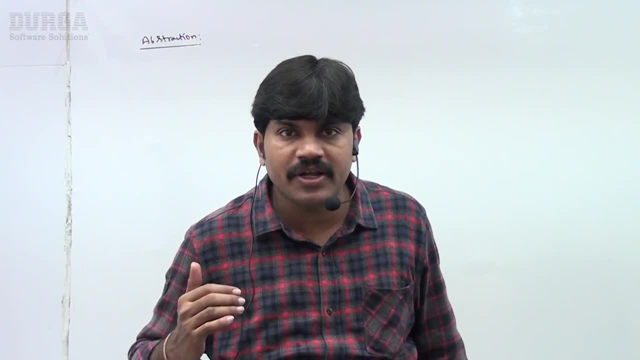 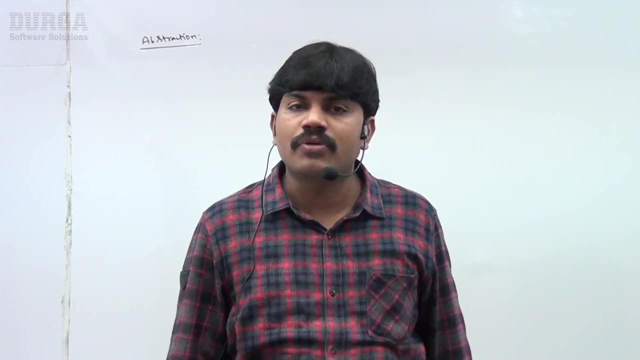 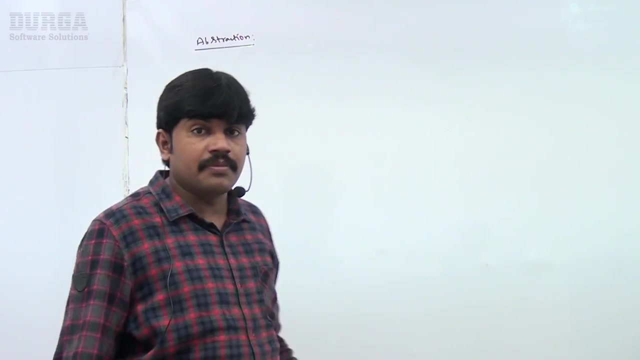 want to highlight my internal implementation. Are you getting So hiding internal implementation? just highlight the set of services. what we are going to offer is the concept of abstraction. Are you getting that? So it's a very important concept, Compulsor while implementing Whoops. 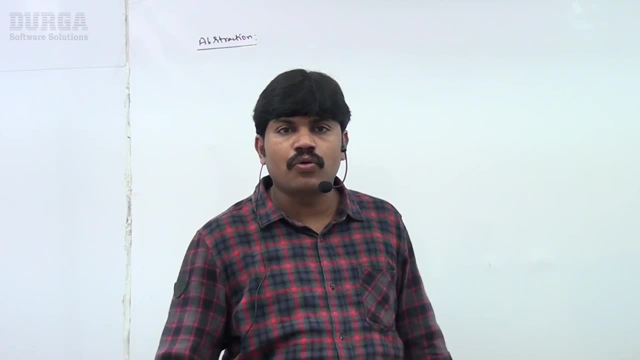 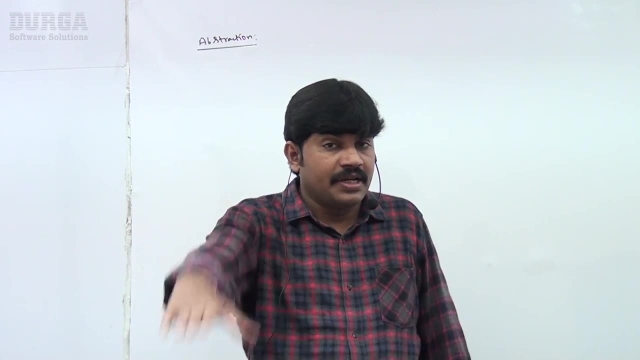 we have to take care, Because if I am going to expose my internal code to anybody, I am giving this information to that person. Then automatically where is the security for our code? That's why So feature must be compulsory required. Hide internal implementation. Just. 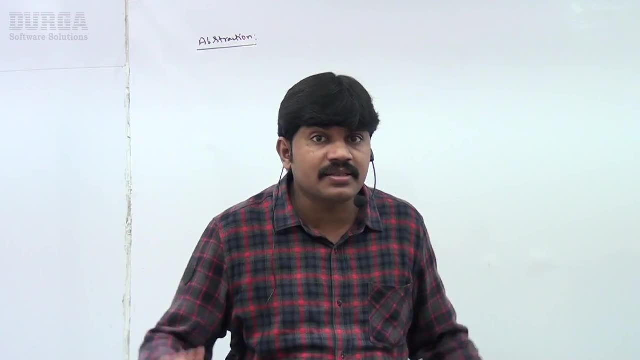 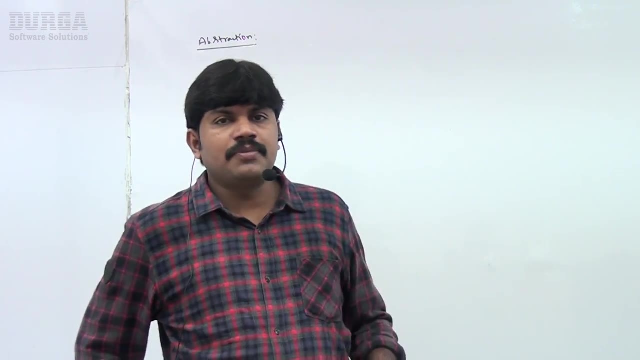 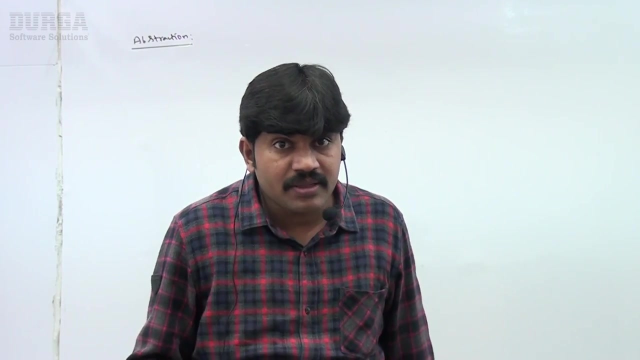 highlight the set of services. what we are going to offer is the concept of abstraction. Sir, best example, best example, sir. I hope everyone in this session- I mean everyone who is seeing this video- used at least once your ATM card Okay To withdraw money ATM. 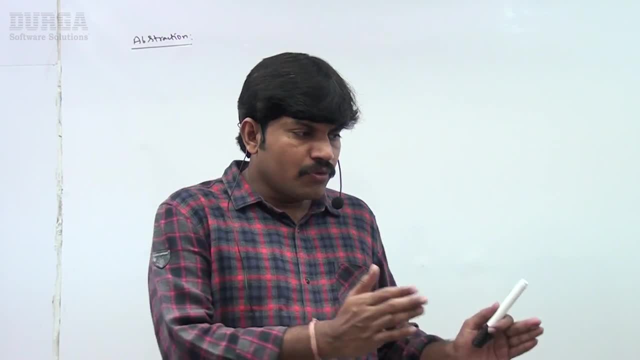 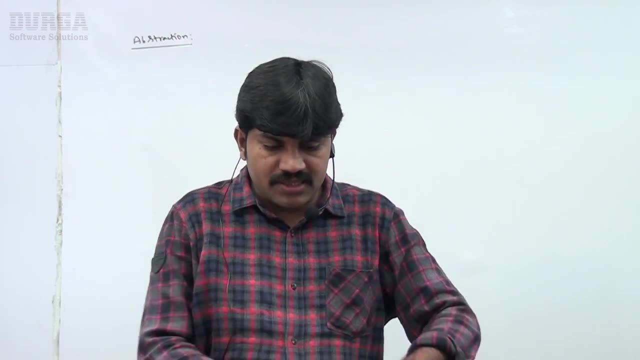 card at least once a month, right, You may be using your ATM card here. Okay, You are, least once you use it, right? so if you go to ATM Center, if you swipe the card, if you swipe the card, then immediately it's going to ask: enter pin number. yes, I'm. 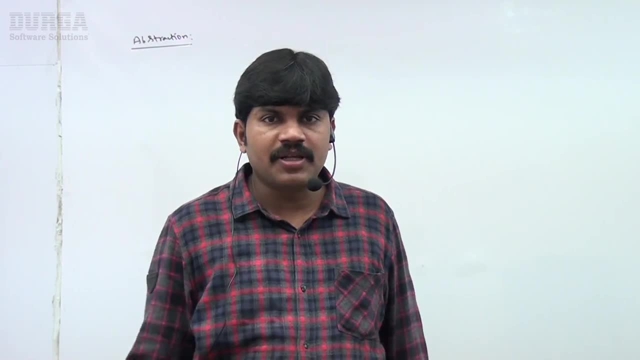 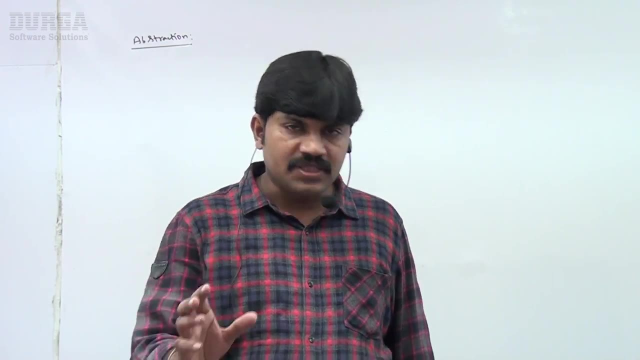 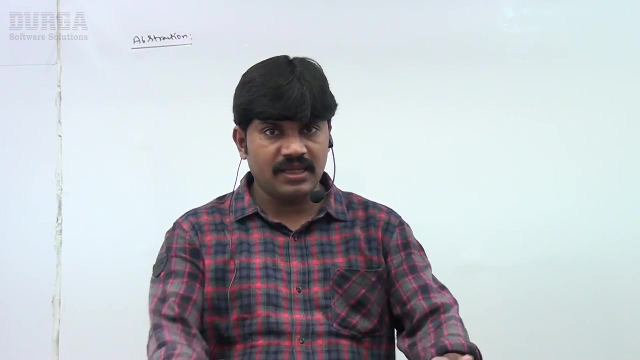 going to enter pin number one, two, three, four. once I enter pin number, then immediately. so which operation you want to do with the operation. click withdraw button from savings account. ten thousand rupees. enter ten thousand, submit now immediately. you are going to get a ten thousand. yes, like this we did several. 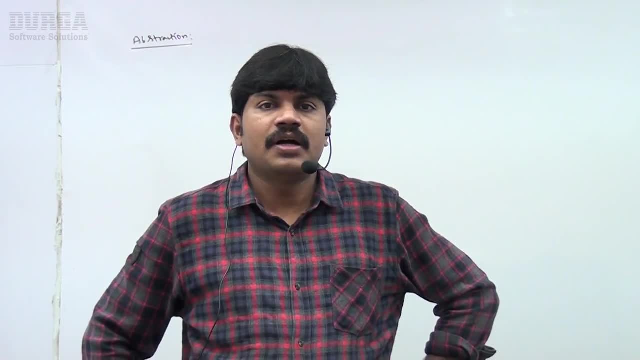 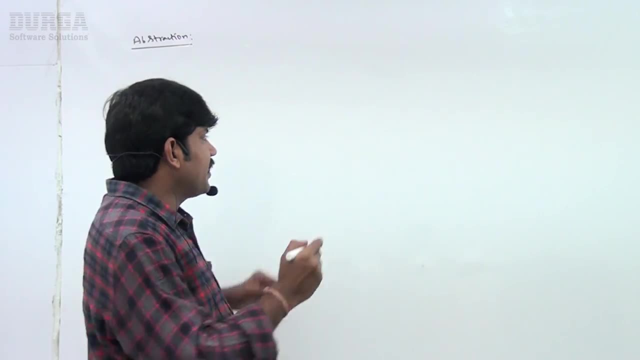 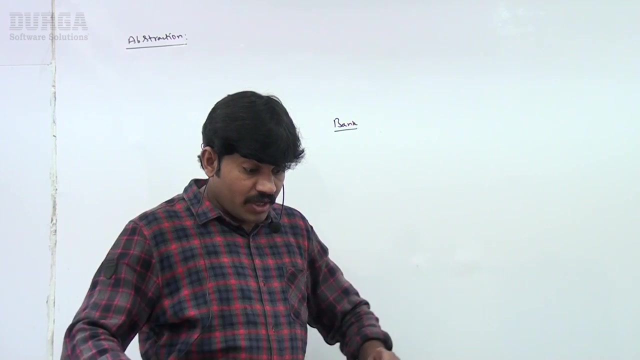 times now in this process, I have several doubts. are there, sir? what I did is one fine day. I went to bank. observe very carefully, sir. I went to the bank near ICC bank or HDFC bank. I went once I entered into the bank on the right hand. 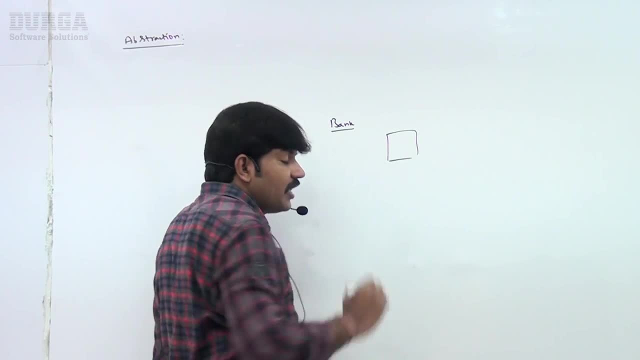 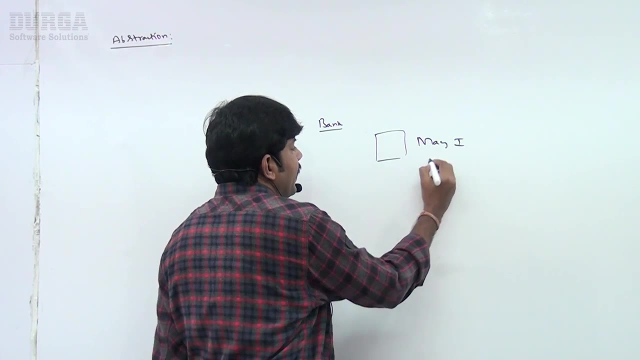 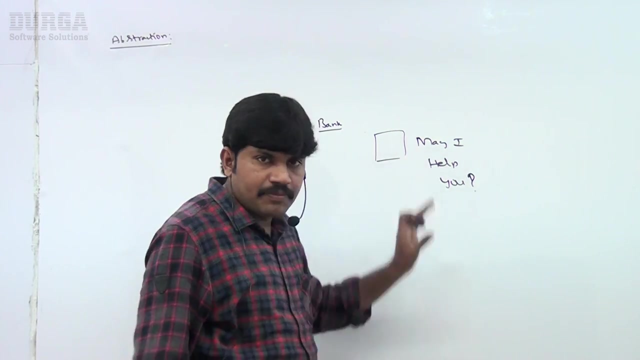 side, you know on the right hand side. so there is one customer care or reception or something like will be there. so may I help you. so may I help you like, sir, there is a one one Center is there, sir. may I help you like one one, sir cabin by. 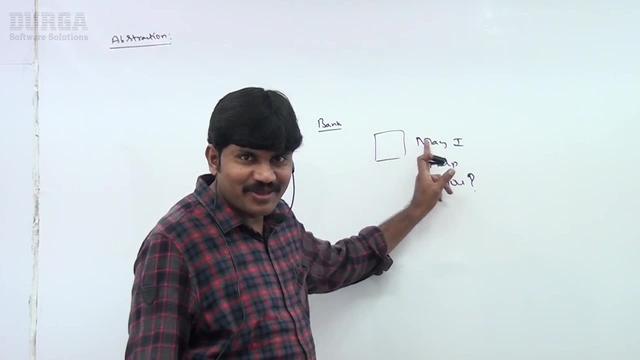 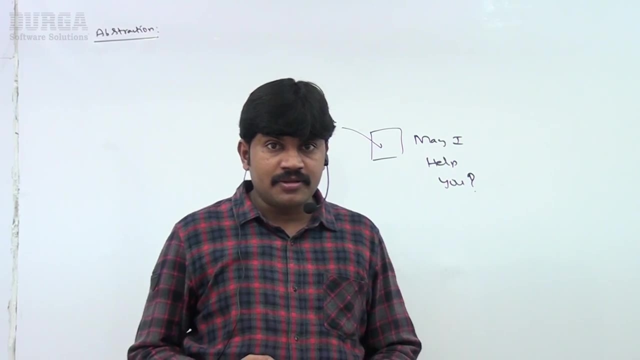 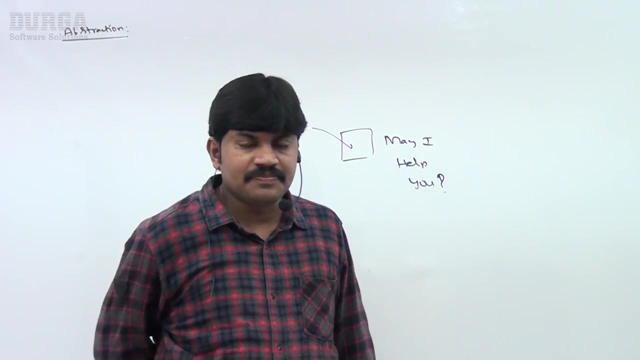 default will be there. very cute lady is going to sit there most of the times. right then I went. I went there, madam, related to my ATM card, my ATM card usage. I have several doubts are there? can you please help like this? I asked this lady- that is information. I ask her many questions- said yes, sir, then immediately. 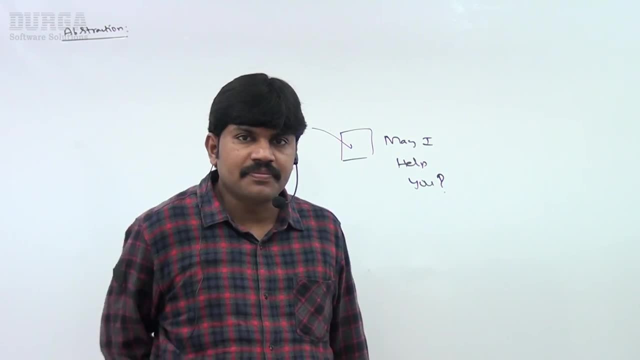 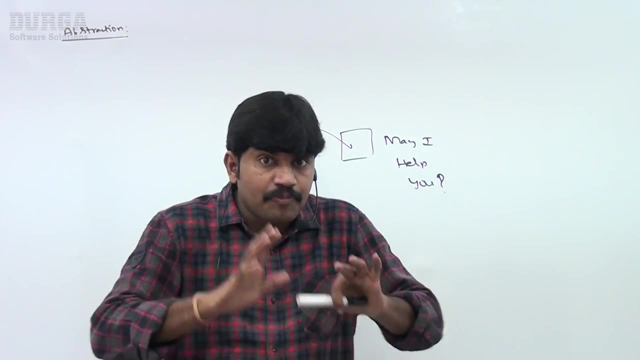 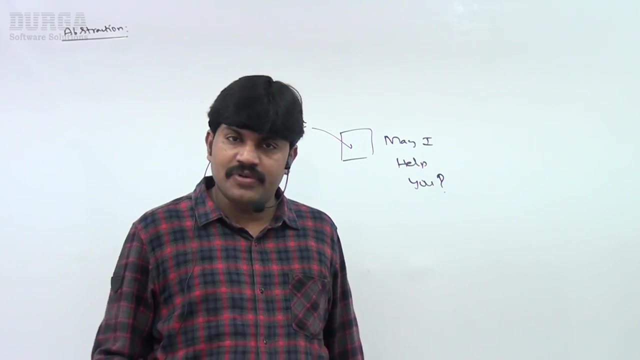 that lady is telling: yes, sir, why not? you can ask you about doubts. I can clarify, like now the first question. I asked her: that lady, madam, whenever I swipe my card, whenever I swipe my card, you enter pin number internally. what thing is happening like this? I asked her then immediately. that lady told: sir you, 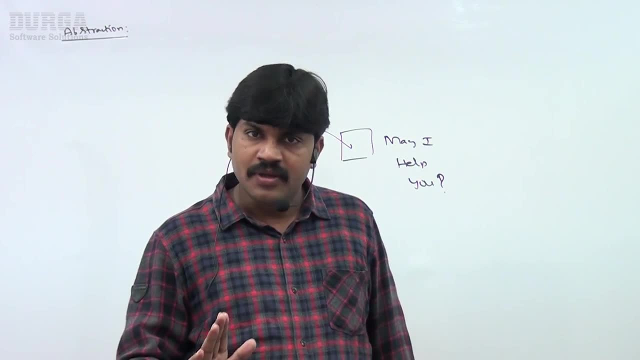 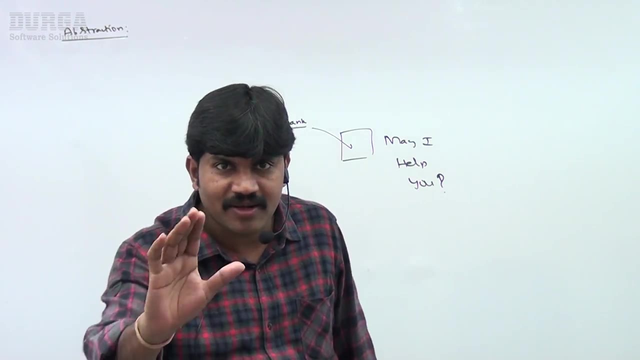 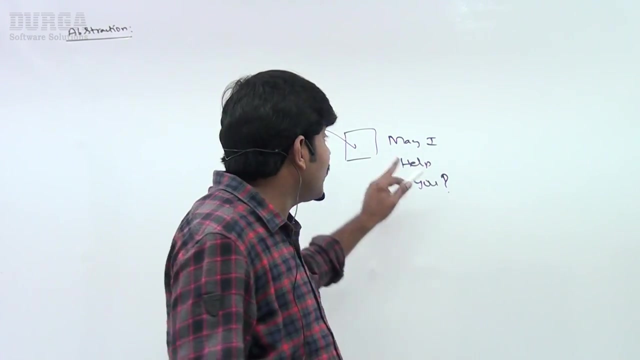 were calling the valuedAond relevant is going to check. our software is going to check to that. I know, I know. but my requirement is, internally, which code is executing? is it Java code or Python code or dotnet code? next, is that a validation, authentication, checking validation. is it happening in the ATM machine or somewhere? 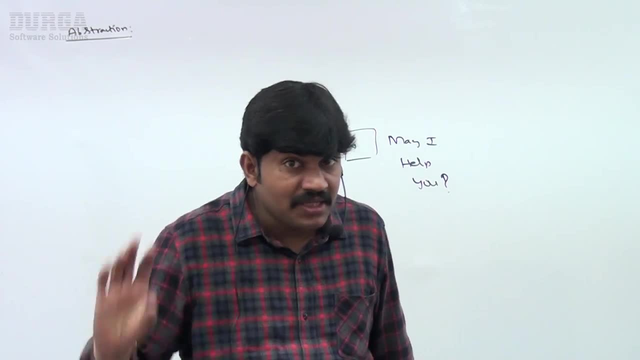 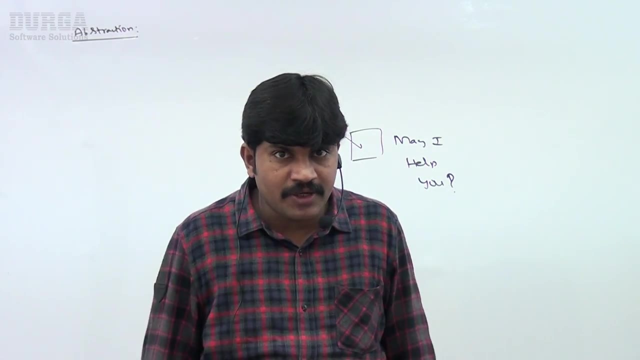 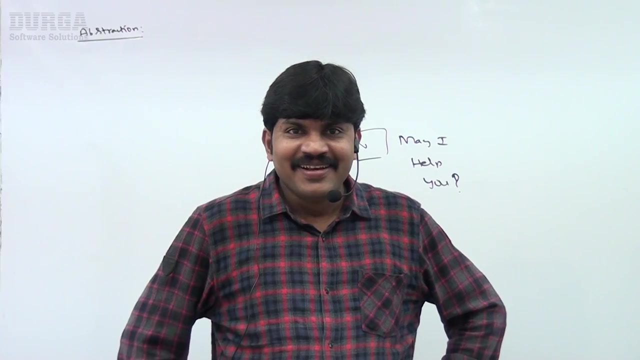 somewhere in the server. if it is happening inside server, okay, where is the location of that server? again, where is the location? what the IP address, what the username and password? next to which SQL query is a triggering? can you please let me know? like this I asked her getting right immediately, sir, if you. 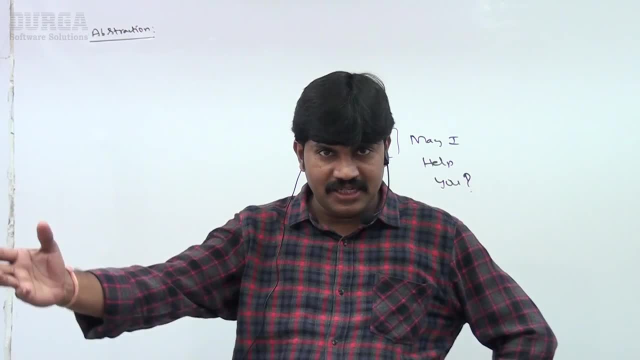 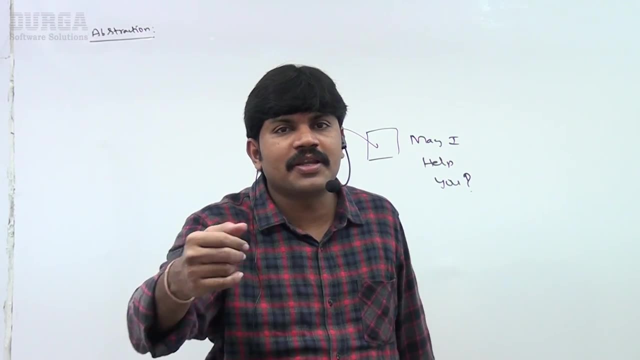 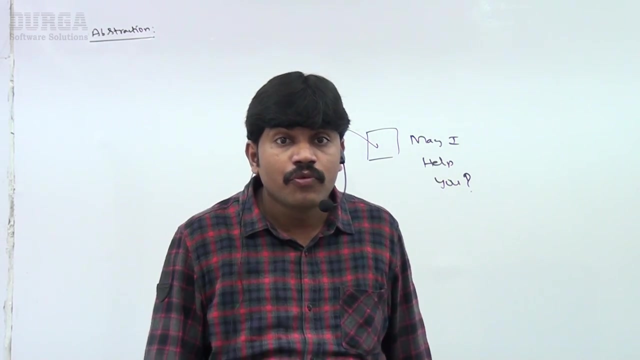 don't mind, just wait here for few minutes. I will call my next level. that person can guide you. like she entered inside, she had a discussion with the manager. those people made a phone call to 100 saying someone came. he is asking about internally server location, IP address and so on. we thought that is the. 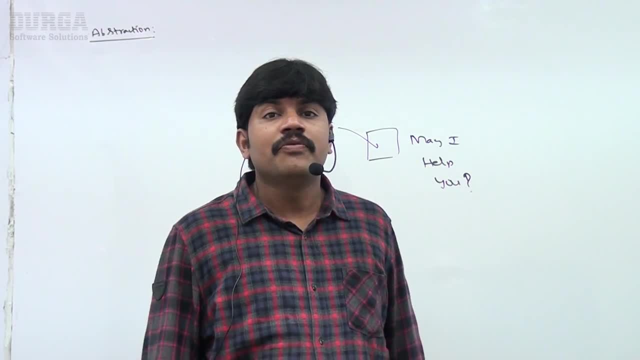 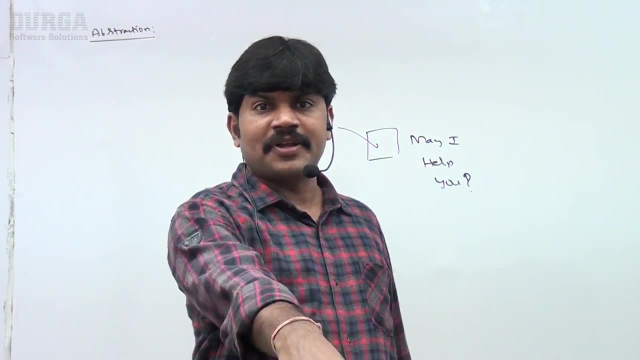 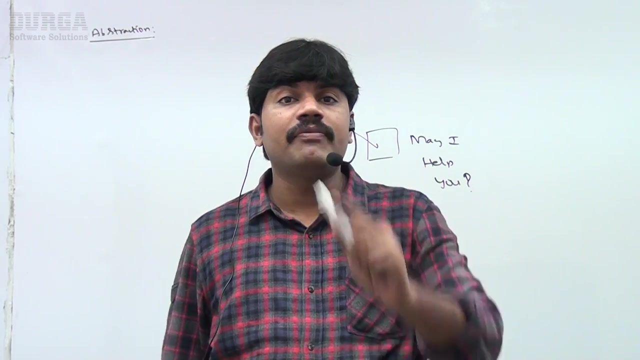 hacker. can you please come? like that, they made it a call to policeman. within 10 minutes, policeman is going to come in front of me not able to get right. so you are the valid customer of the bank. you have already ATM card, sir. you can able to use this card, but you should not aware. 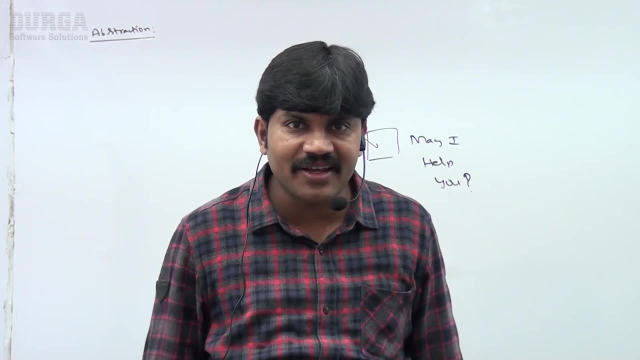 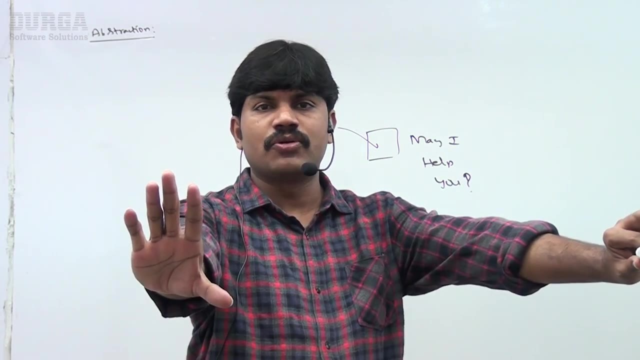 internally how that functionality is implemented. are you getting right? so if you want to validate, enter, enter swipe the card, enter pin number. that's all. internal validation is going to be happen. hurry, how the validation is going to be happen. sorry, sorry, sorry bank people. they never going to highlight their internal. 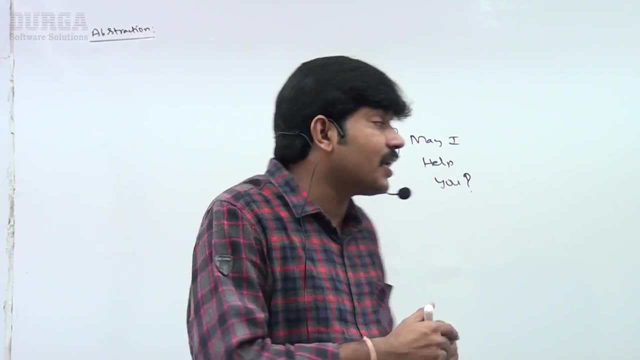 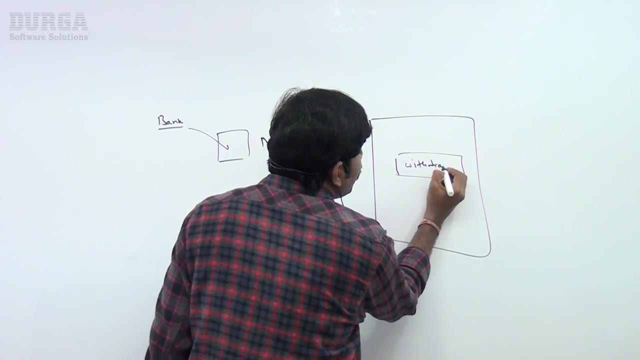 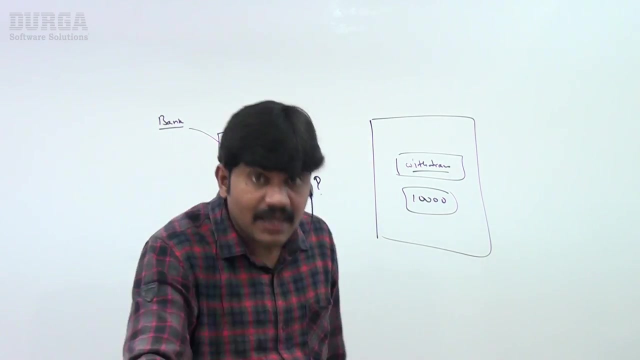 implementation. okay now, if you, if you click with the drop button, if you click with the drop with the drop button, sir, I'm taking with the drop button, if you click with the drop button, if you enter ten thousand, so you will get the ten thousand. so, internally, how this functionality is implemented? which SQL? 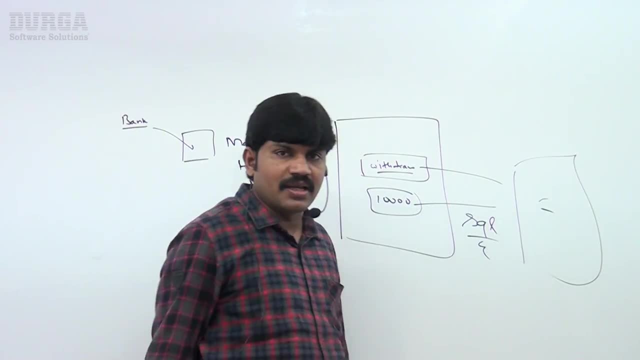 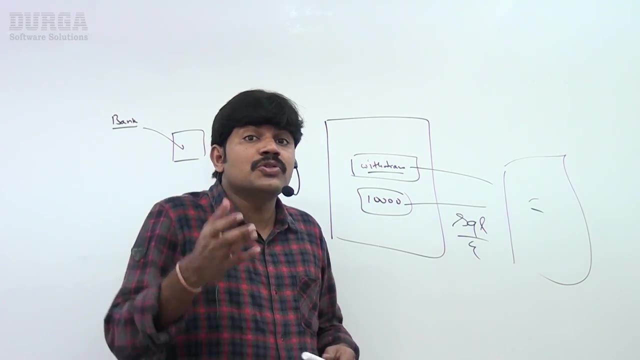 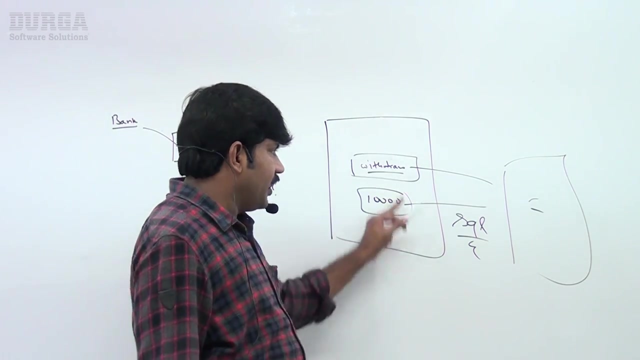 query is executing? where is the database server is locating all these things? bank people they never going to highlight. are you in the position to understand, right? so this is the? so this type of feature is nothing but abstractions. are bank people through atm gui screen are getting 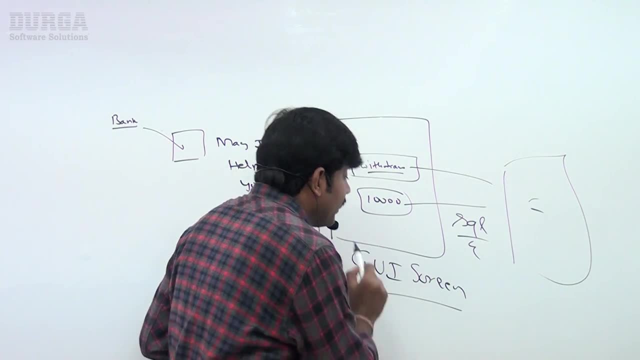 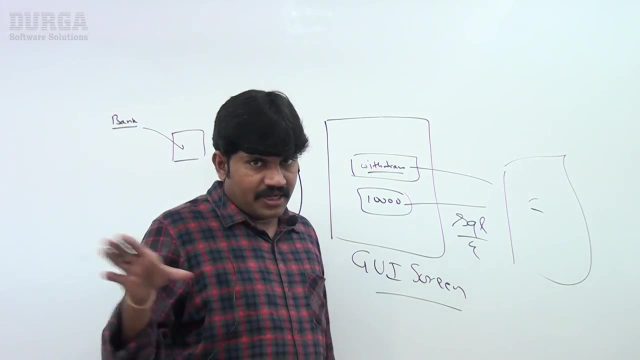 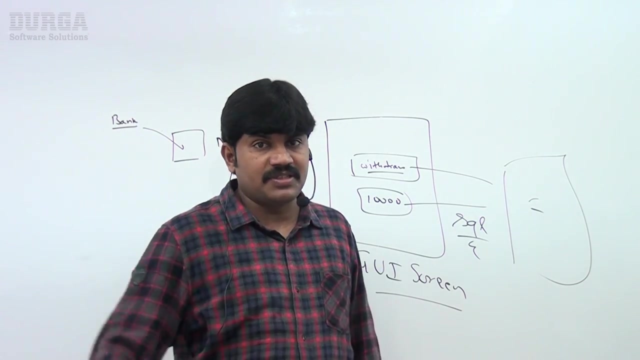 through atm gui screen. they are going to highlight, they are going to highlight the set of services, what they are offering. so i say, say bank atm center. they are going to tell, even very recently they got one world world, sir. mini bank atm mission itself is nothing but mini bank counter, like they. 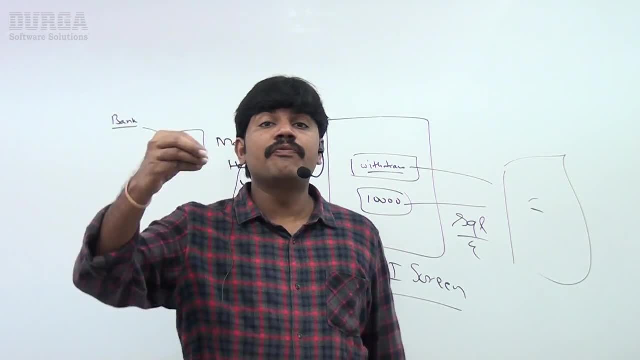 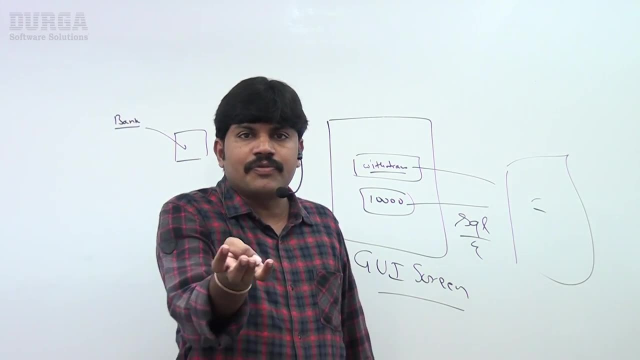 got some award. they are going to tell boss these are 15 services we are going to offer through atm mission. like i say, say, bank people are going to tell very proudly. so with the drop facility is there? deposit facility is there, next to fund transfer facility is there. so request for 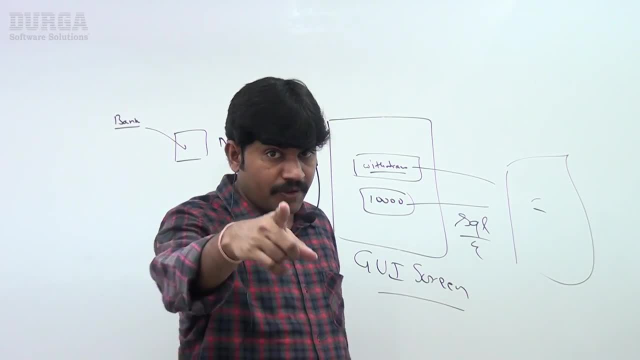 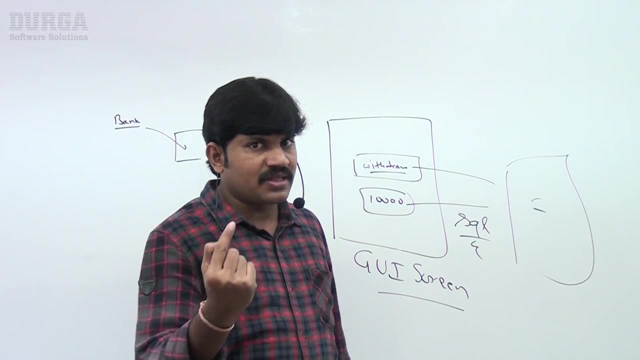 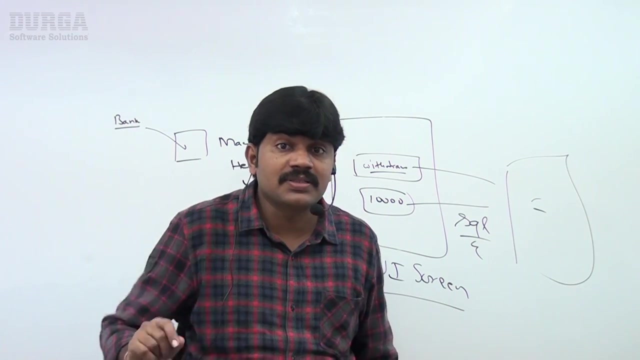 checkbook, like there are multiple services you can able to get from atm mission, but but internally, how the services are implemented? at least one service also they never going to highlight. are you able to identify? are you able to understand the point right? so this concept itself is nothing but this concept itself is nothing but. 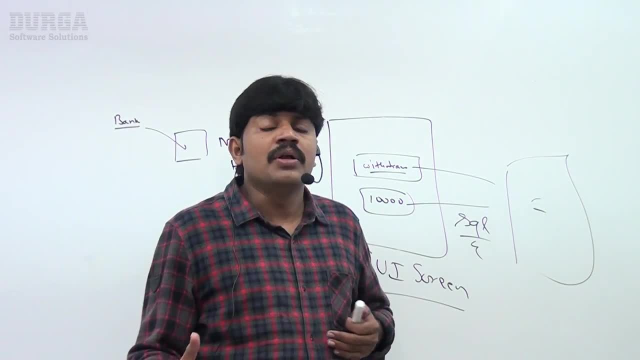 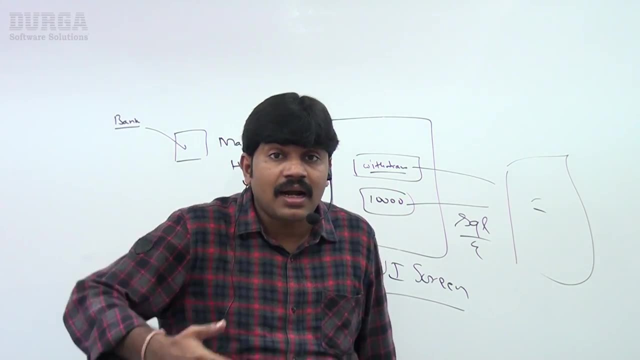 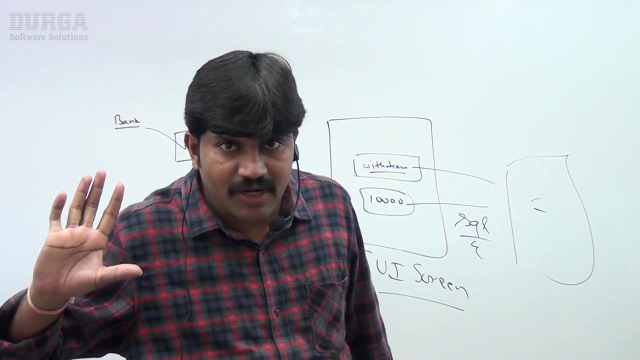 abstraction. so in our coding, also compulsor, we have to maintain this type of feature, hide the internal implementation and highlight the set of services. what we are going to offer either concept of abstraction, is it clear for all operate. so by using GUI screens, interface concept, we can able to 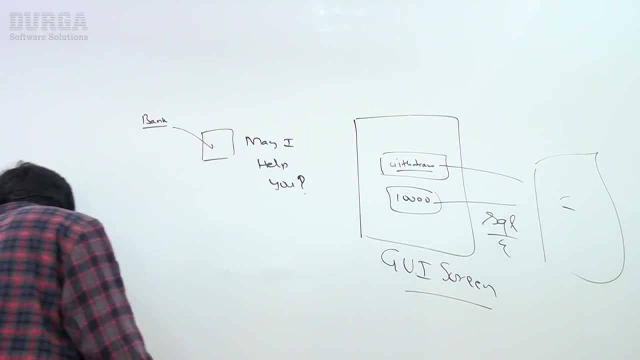 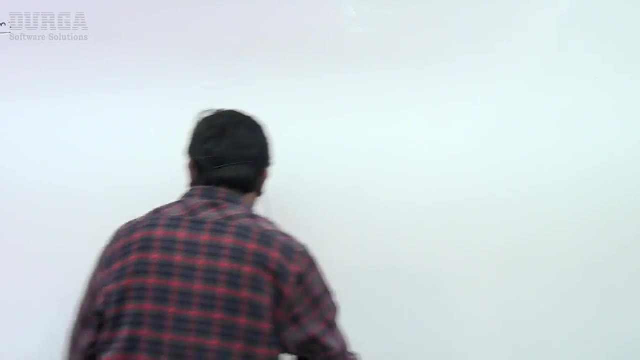 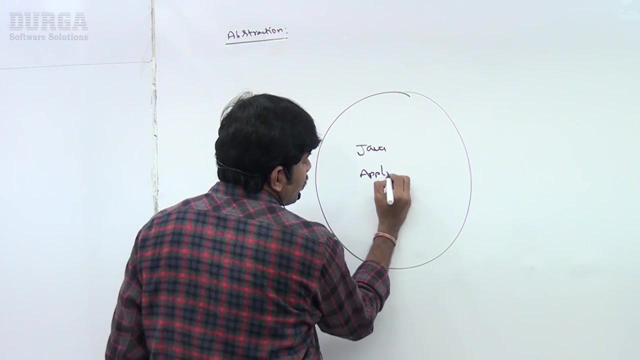 implement abstraction, sir. best example: get a programmatic level. just observe this one. so suppose I want to develop, I want, I want to develop a Java application. assume that it is the Java application application. right now there are some services are available with the draw funds, transfer, deposit. 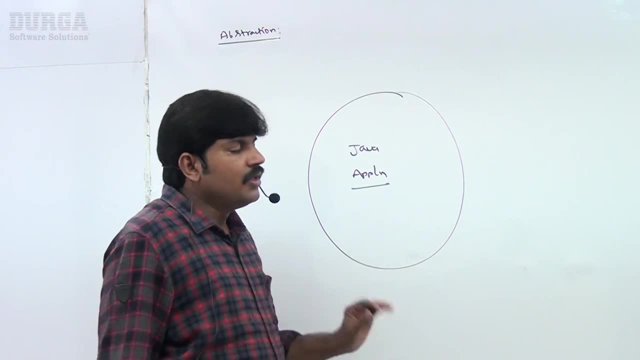 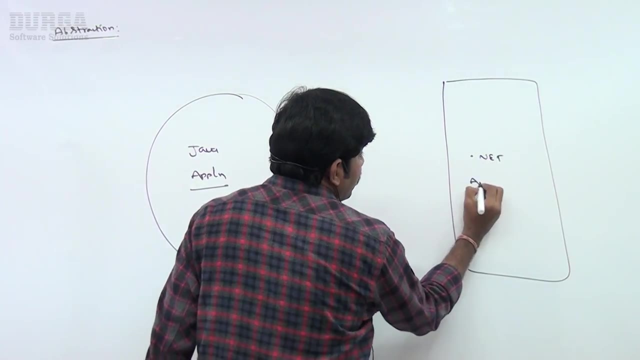 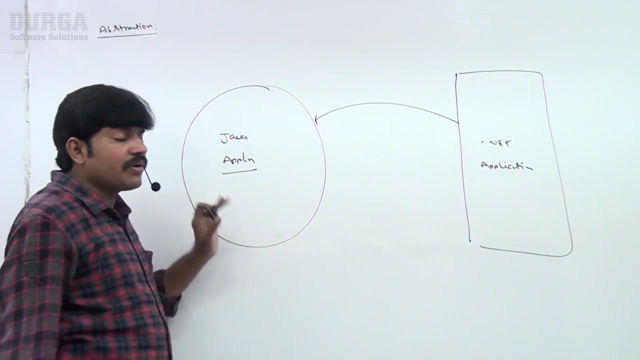 etc. it like there are several, several services are available right now, sir, a ui based application, dotnet application, dotnet application wants to communicate with this dotnet application wants to communicate with our java application. so, array, if you want to call, withdraw if you want to. 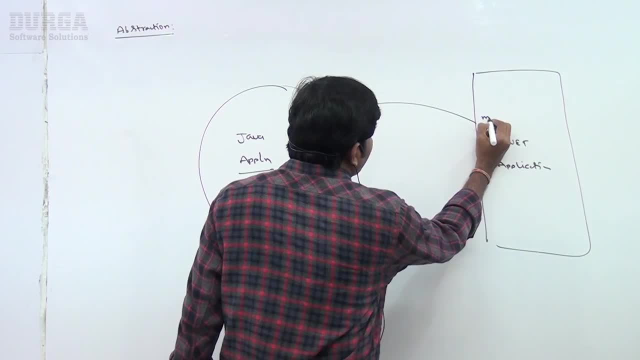 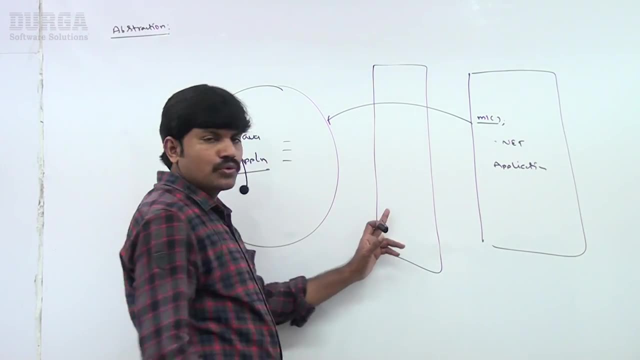 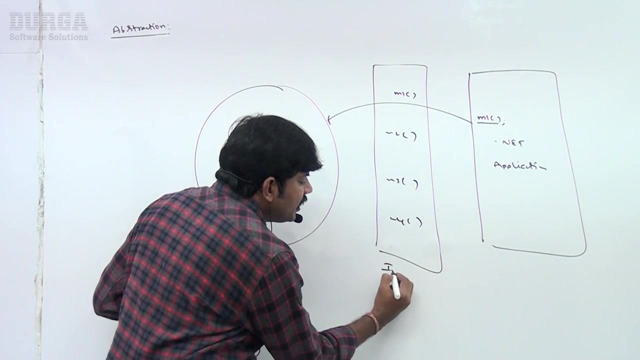 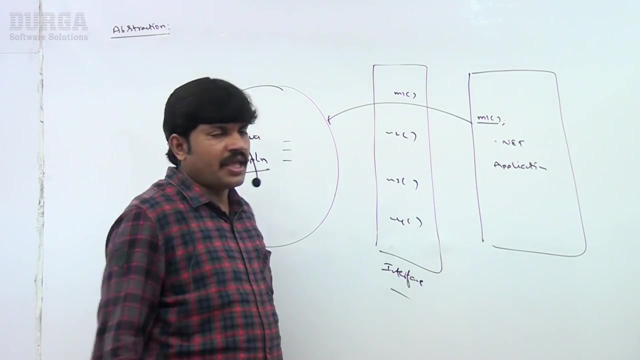 call withdraw, just uh, you have to call from your code m1. okay, in the middle, in the middle, i will expose all my services through some interface, sir, m1, m2, m3, m4, something like it is. an intrapiece regarding itself is interfere. dotnet person has to call. m1 method has to call. 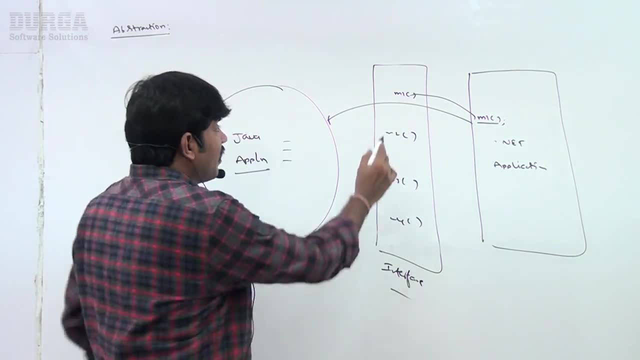 elemente internally. whenever this person is calling m1, you need to though thisCharacter should callnet method. you do this, you do this. WTO call: call Water, Mozart, dotnet. and do you have a translation of m1 phone callrin's code For this method? the service should help you with your n1. E-mail with meように. the book is not Cavalry n all the way. you have some work to do With Windows Face cp. Wgl Over sentenceว tend to flow n all the way через a code errorsand called未. there should help checking n1 at the end. you should alwaysしか نہ you. you should consult with Chrome and do not click on the browser internet. 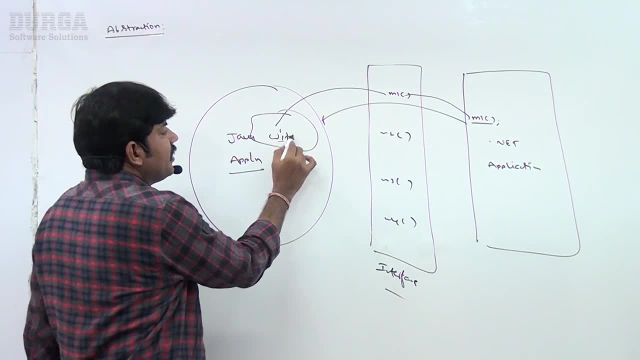 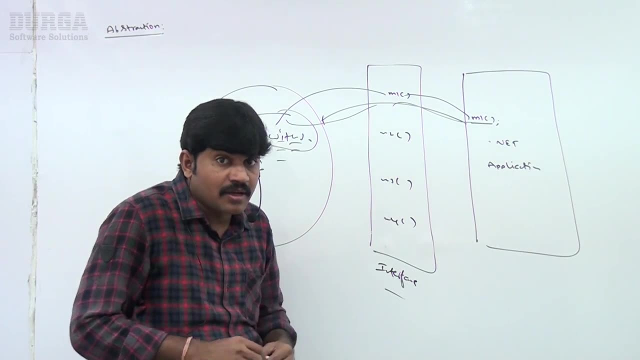 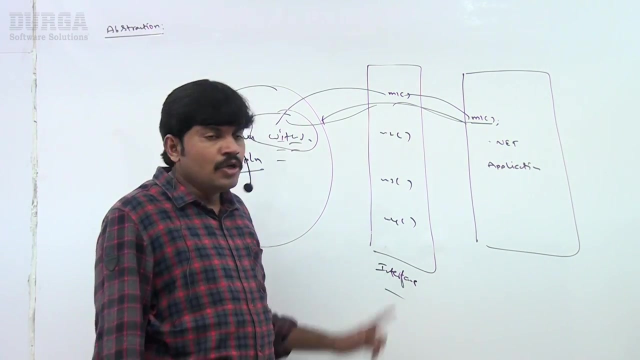 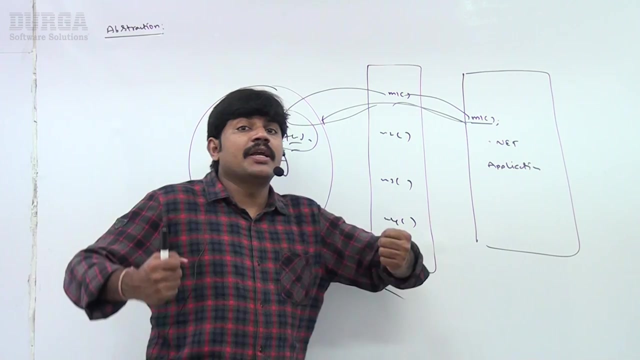 internally which method is going to execute? maybe some withdraw method is going to execute the required result we are going to offer to this dot net person. we never going to highlight internally this application, how it is implemented. are you able to understand, right? so because of this abstraction, because of this interface concept, two different applications also can communicate with. 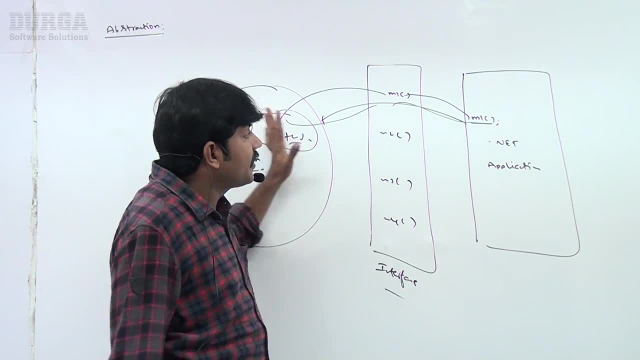 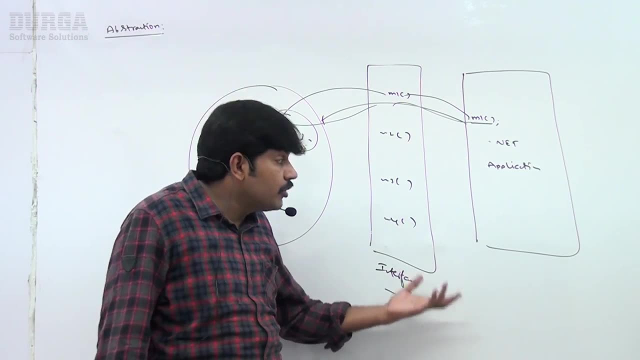 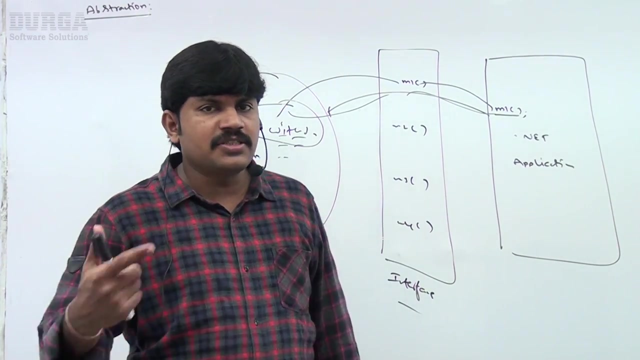 each other. yes, can communicate with each other without highlighting our internal implementation. everyone can able to understand. so abstraction is how much important in our day-to-day coding in real time. please make sure you should aware. so if the interview person is asking what is abstraction, can you please tell what the answer you? you can able to tell, yes, friends, what answer. 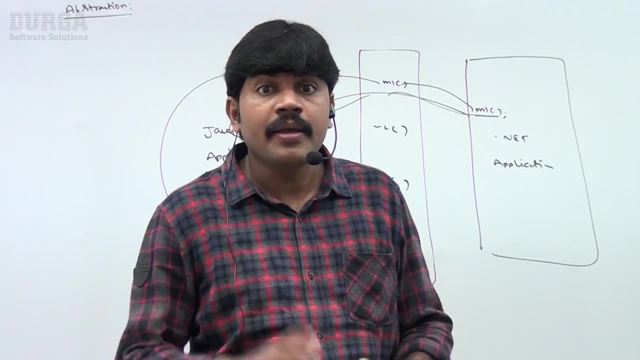 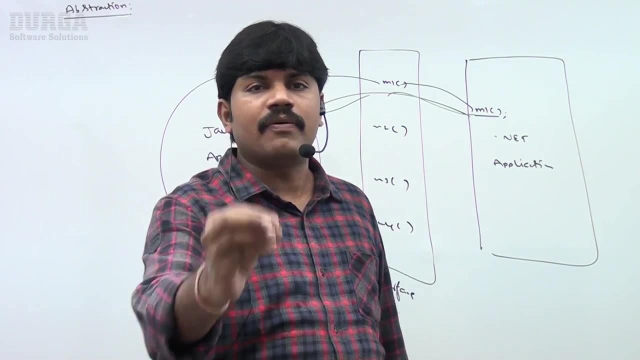 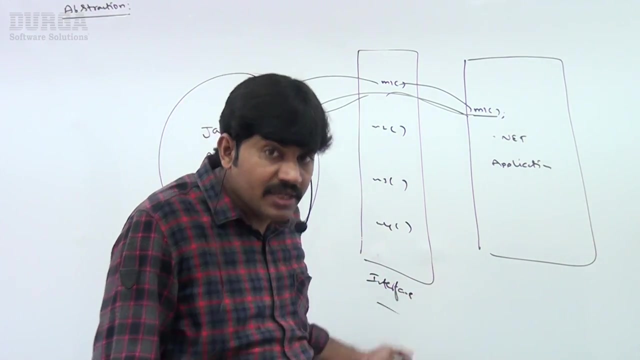 you can able to tell. you can. you can tell what answer? okay, hiding internal implementation. just highlight the set of services. what we are offering is the concept of abstraction. okay, clear. but using some gui screens, interface concept, we can able to implement abstraction. okay, sir. now what are? 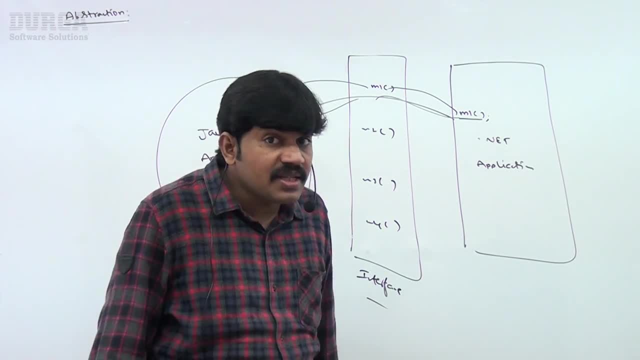 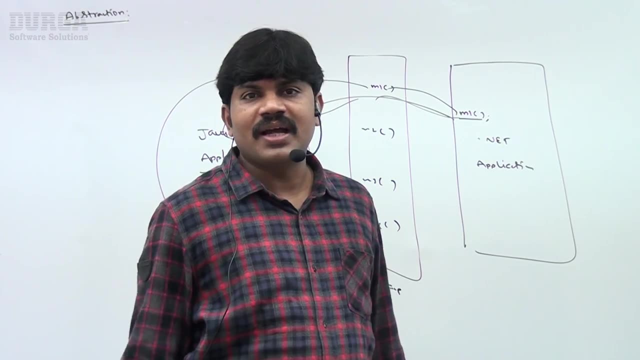 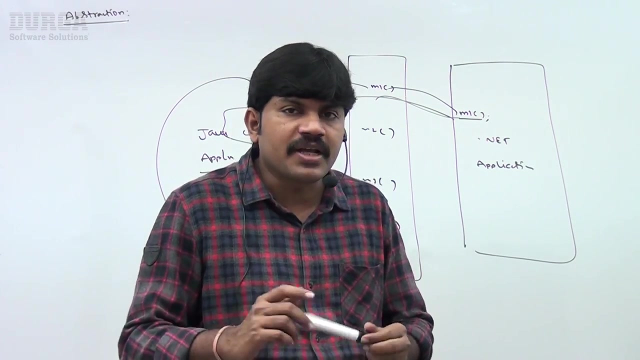 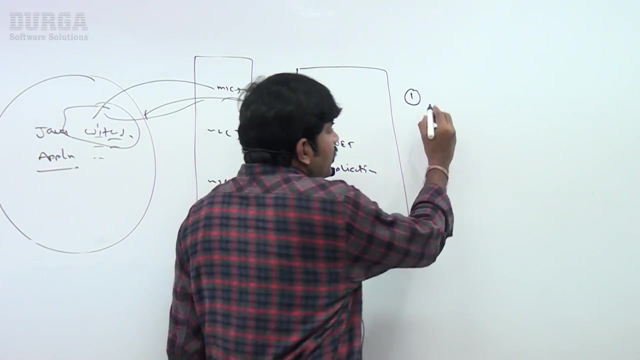 various advantages of abstraction. so best example for abstraction is atm gui screen bank. people are going to highlight several services, but they never going to highlight internally how the services are implemented. okay, so what advantages are there because of abstraction? so the first advantage right. take very special care. what the first advantage, right. the first. 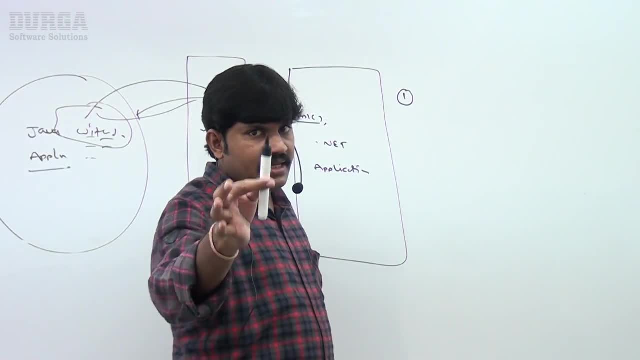 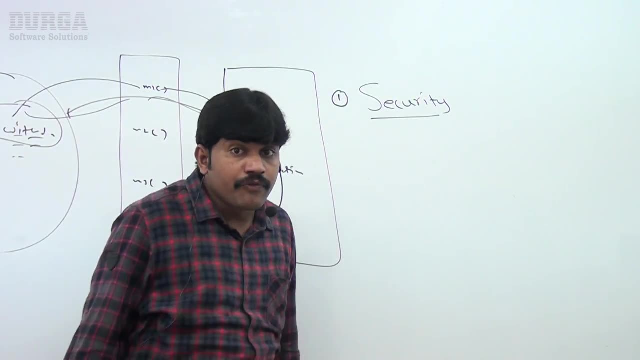 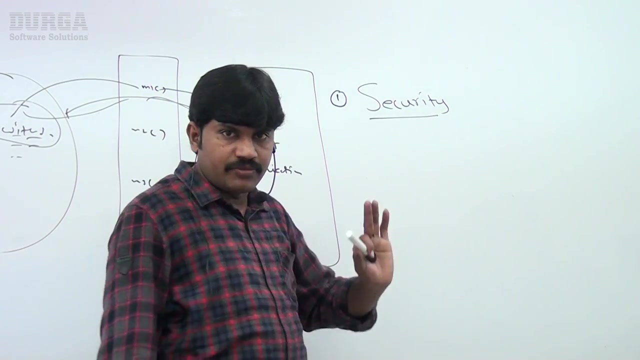 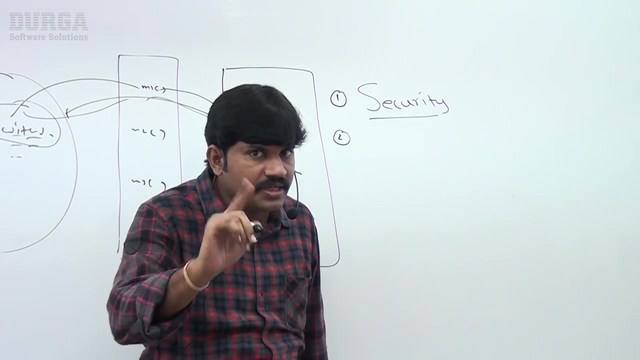 advantage is: wherever hiding is there the biggest advantage? what we are going to get is security. are getting wherever hiding? is there the biggest advantage? what we are going to get is security is the biggest advantage, right, okay, like the second advantage. what we are going to get. the second advantage is, sir, very simple. 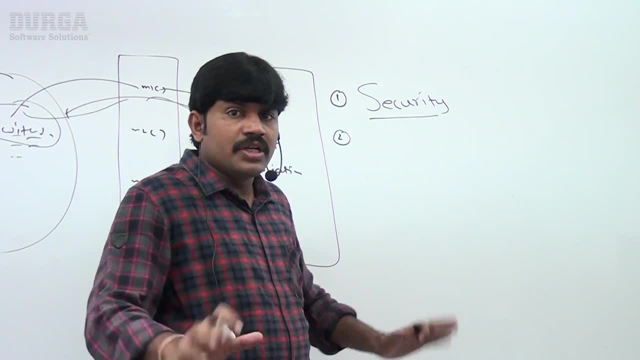 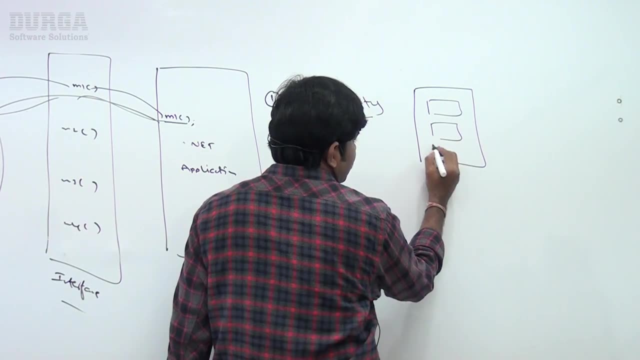 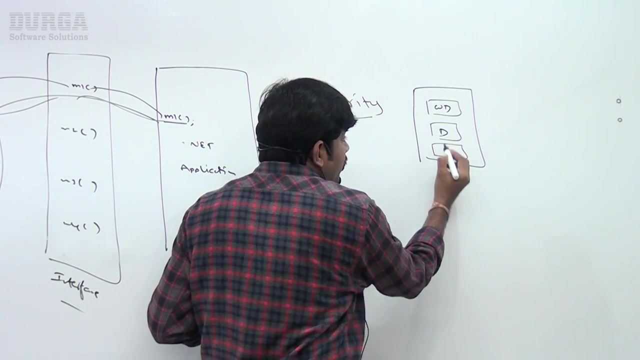 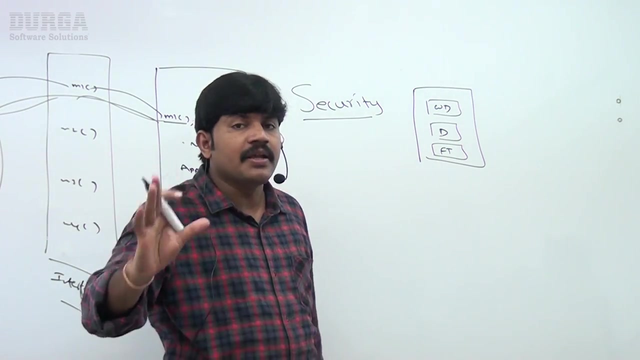 outside person don't know about internal implementation. sir, atm mission- atm mission- gui screen contain some buttons, that's all. we never highlighted internally how these withdraw facility, deposit facility, funds transfer facility implemented. i never going to highlight so. outside person doesn't aware internally how my services is implemented. that's why, first thing, 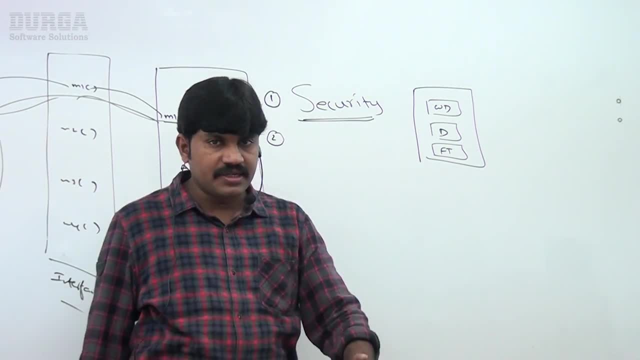 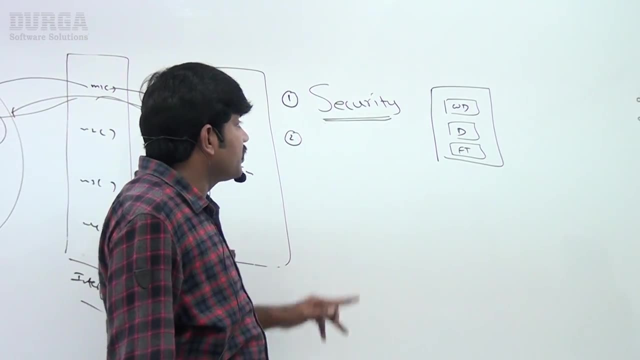 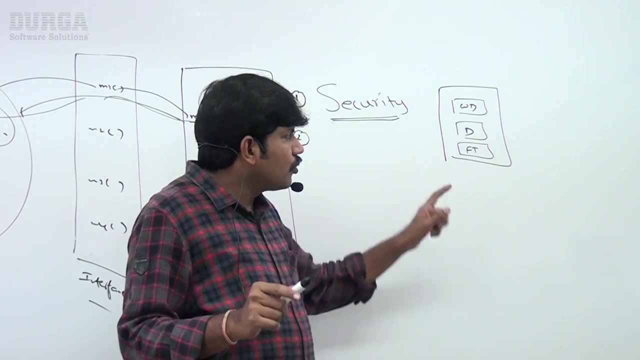 security by default. we are going to get first biggest advantage right now. second biggest advantage: what we are going to get. he is very, very important. points are take a bit special care. second biggest advantage: what we are going to get is suppose tomorrow this functionality already implemented, admitted by Parasite. 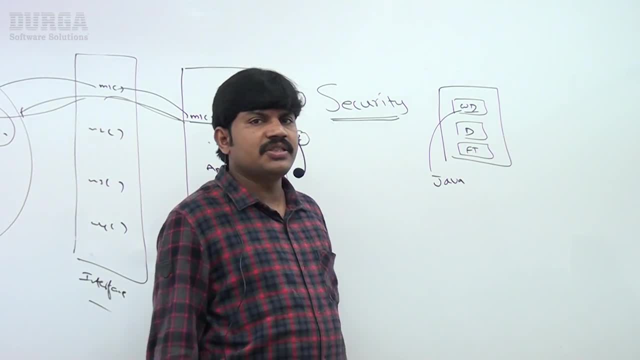 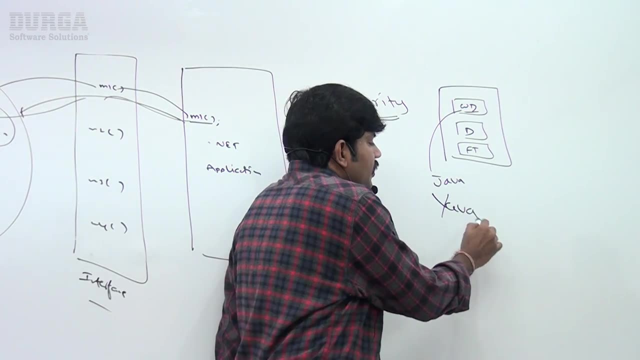 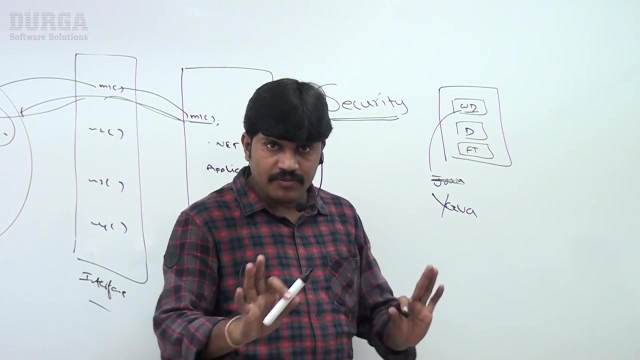 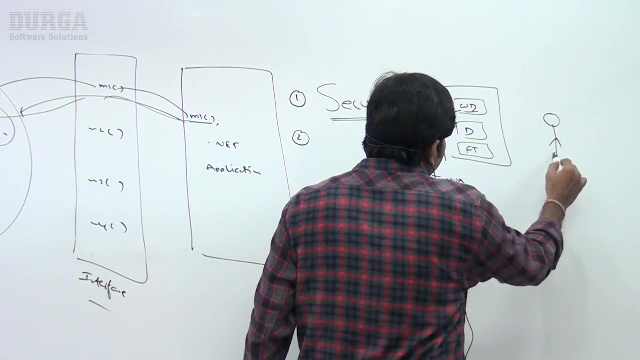 using java, i thought that java is not good, performance wise. okay, a new language came, java language came. i want to replace this java functionality with the java functionality. okay, internally i performed that change, but gui screen is always same. gui screen is always same, sir. now, end user, whenever you click withdraw, earlier, java functionality is executed, but now. 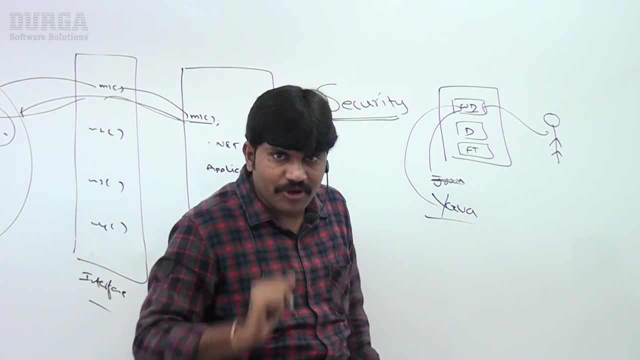 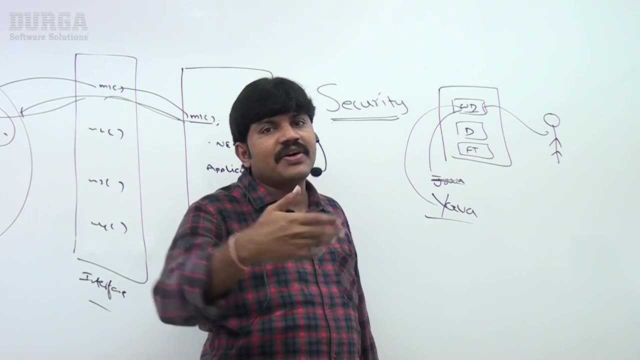 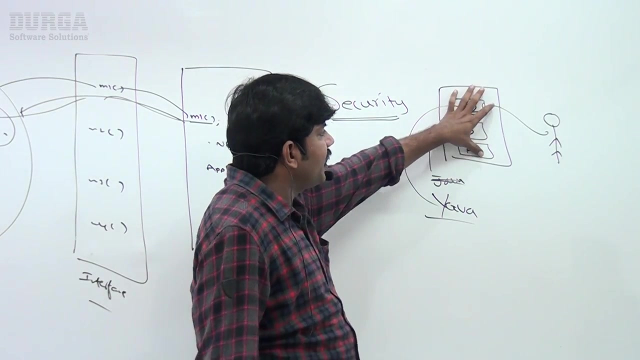 onwards. it is java- functionality is executed. now the point is, without affecting end user, we can able to perform any changes in our internal design are getting right, so we can able to change it technology itself by maintaining same ui screen. so either any effect on the end user. 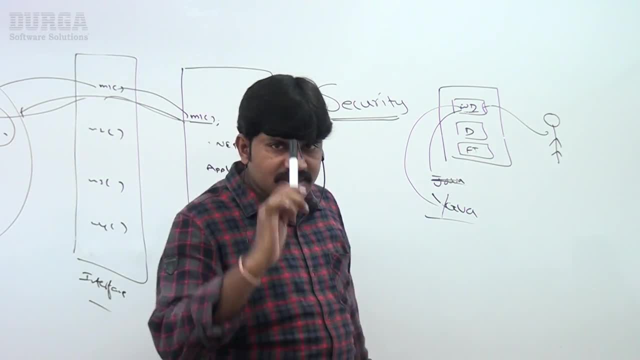 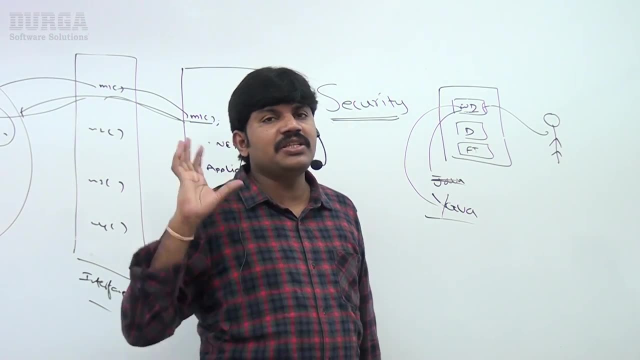 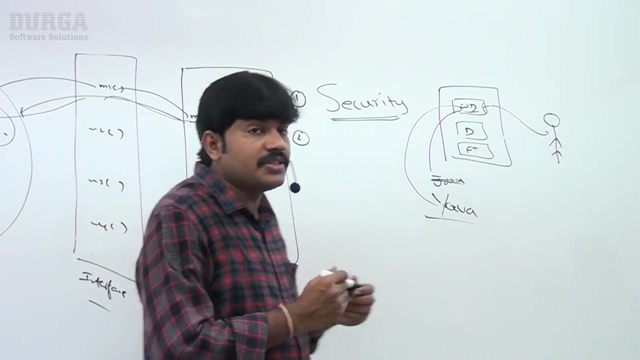 no effect. no effect because end user what is seeing is always the same, but internally, how that functionality is implemented, yes, we can able to perform any changes. that's why, if you, if you are following abstraction, if you are implementing abstraction, the biggest advantage is, yes, enhancement will become very, very easy. are you getting? 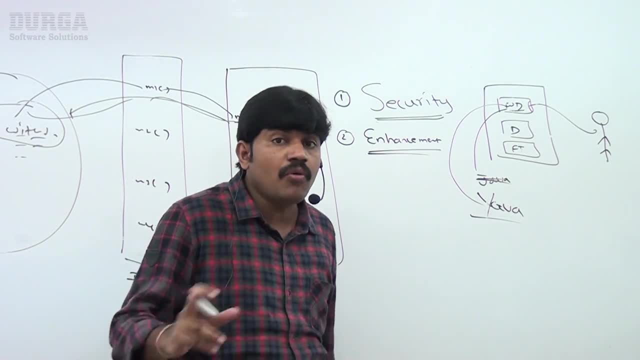 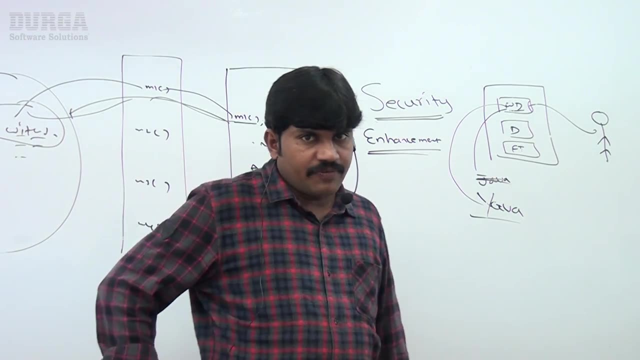 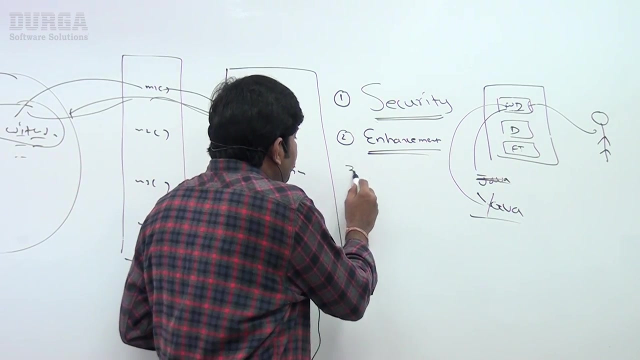 enhancement will become very, very easy without affecting end user. happily, we can able to perform any type of changes in that clear for you. are you in the position to understand, right? that's all. this is the second important point. now the third point. take very, very special care, sir. this is the second. 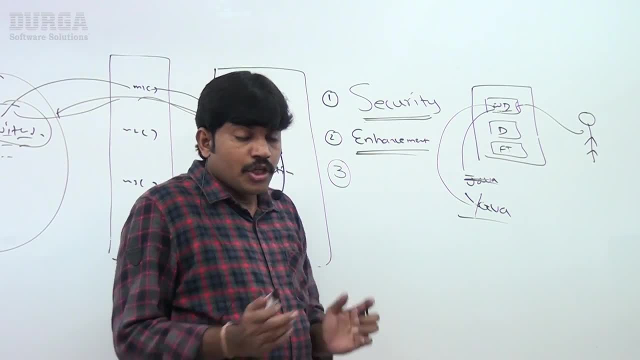 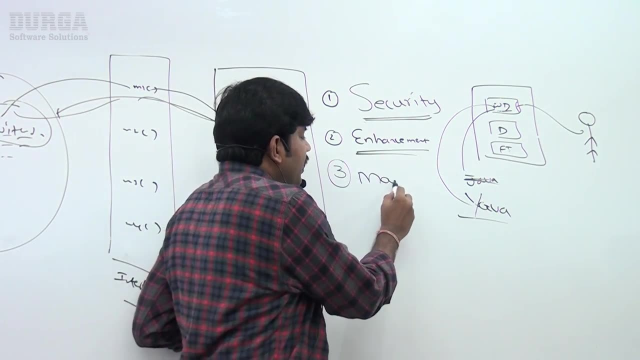 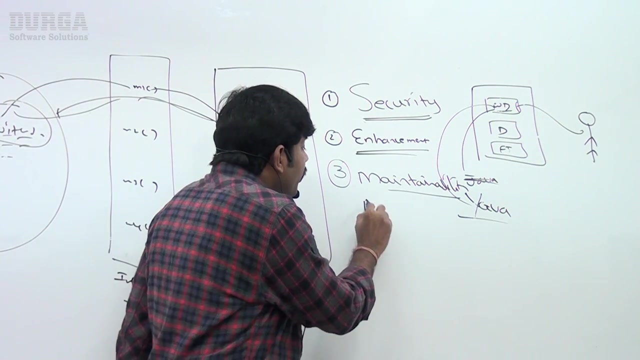 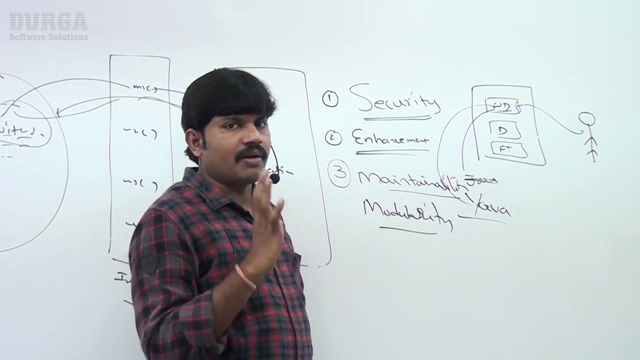 next, if abstraction is there, if you are not going to highlight your internal implementation to the outside person, okay, maintainability of the application is going to be improved. maintainability of the application is going to be improved. modularity of the application is going to be improved, sir. okay, so compulsory. while developing the code, while developing the programming, we 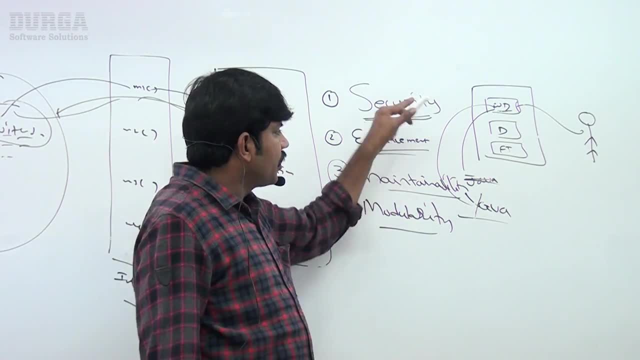 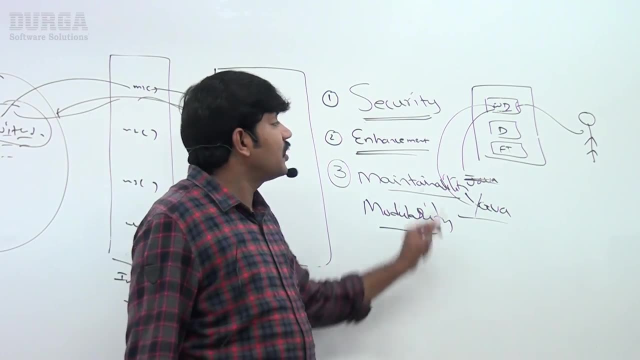 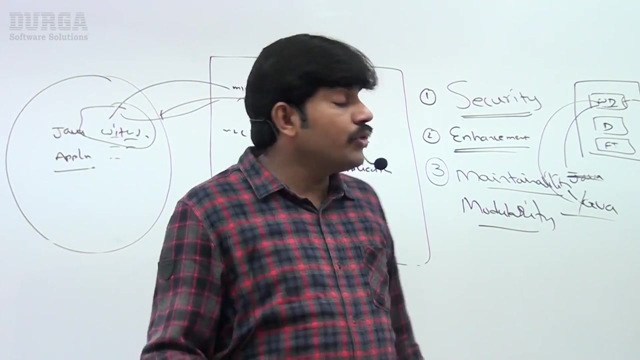 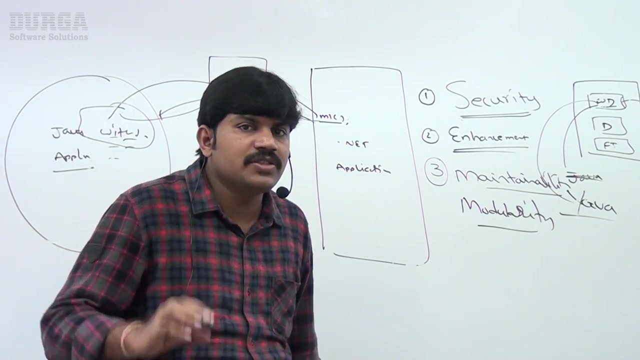 should evade abstraction. so security the one advantage, enhancement is the another advantage. maintainability of the application, modularity of the application is going to be improved. that's all getting the basic idea. what is abstraction? what advantages are there? how to maintain the application? okay, you can implement abstraction by using interfaces, concept gui screens: like by using interface gui.